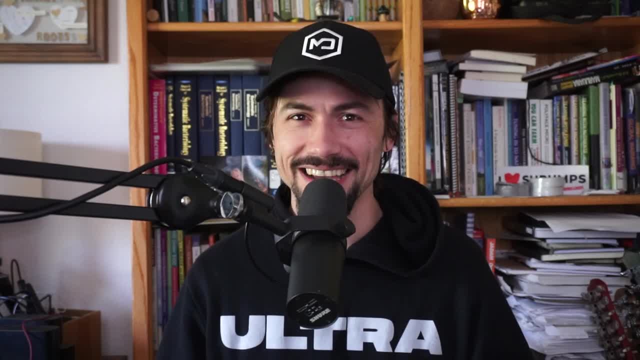 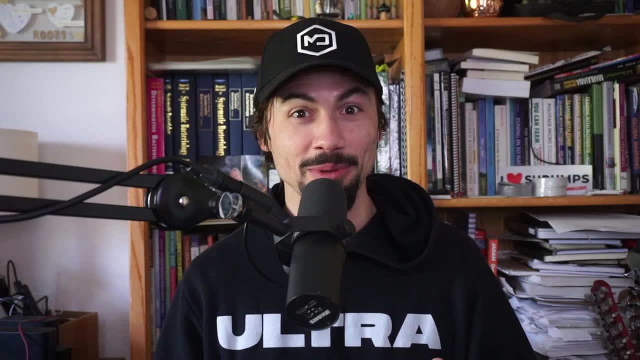 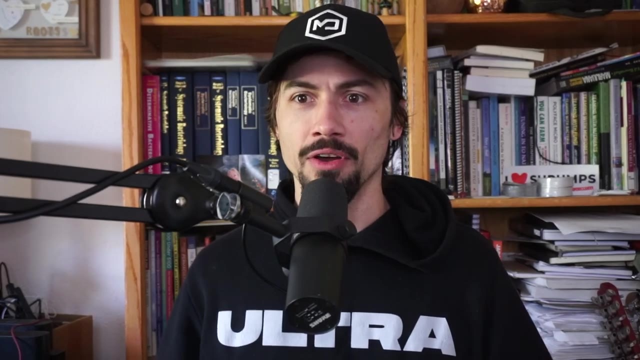 Hey everyone. it's Matt Powers- author, educator, citizen scientist, seed saver and family guy, and I help people all over the world to live more regeneratively And I want to show you something, something that, until I saw it, I hadn't seen before. I've heard of, but I've never seen any. 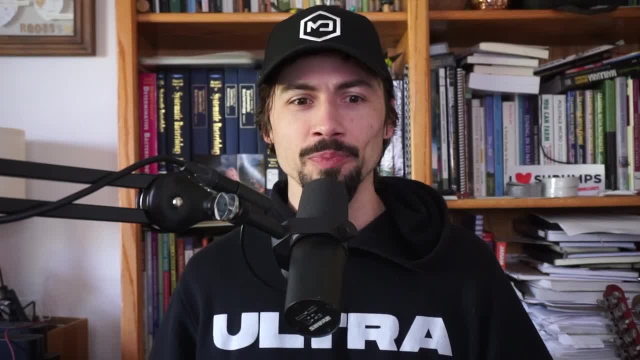 of the people who told me that show me an actual picture. I mean, we've all heard of the soil food web. We've all heard of trophic cycling. We need the nematodes there, We need the protozoa there. 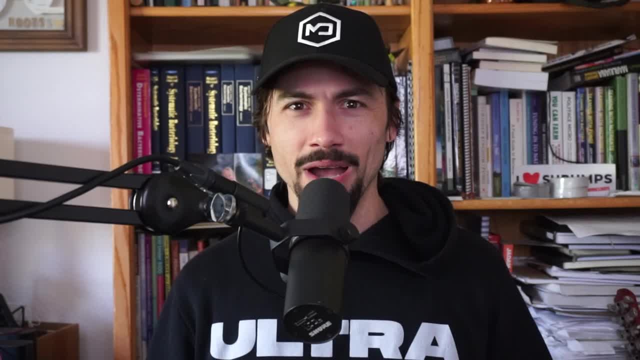 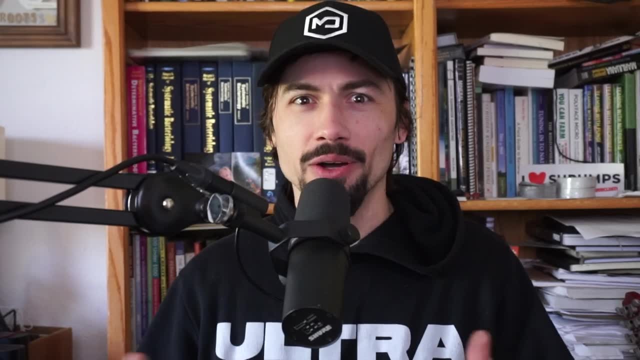 This eats that, that eats this. But have you ever actually witnessed some of these things? And you know a few of them? like you know, bacterial feeding nematodes are so easy to see- Everyone's kind of seen- that There's lots of footage of that on the internet. Not talking, 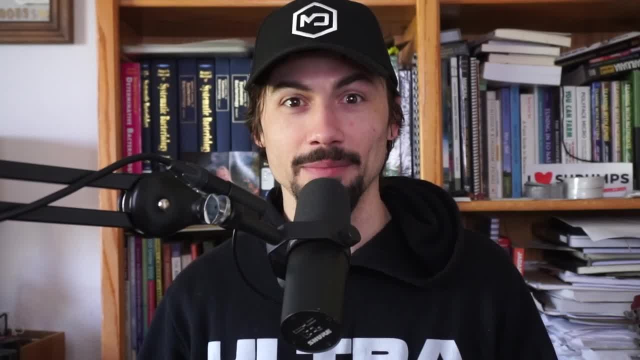 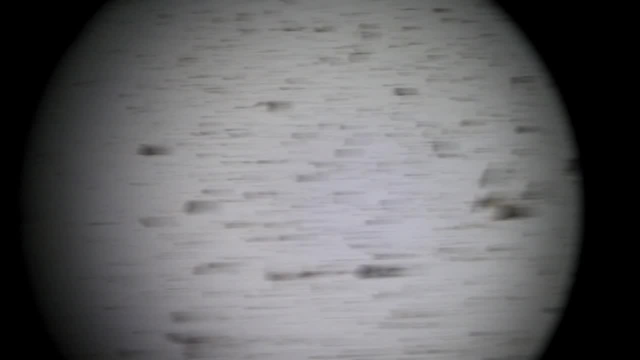 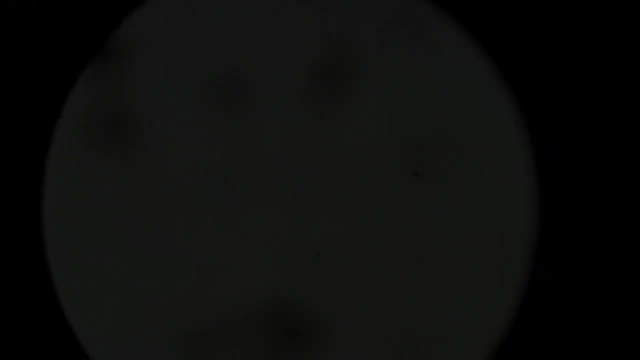 about that. I am very specifically talking about this. Now you can see from here that there's something there, And then let's zoom in. You're like: oh okay, Large testate amoeba, That's not so well, wait, what's? do you see it? Yes, It's moving. 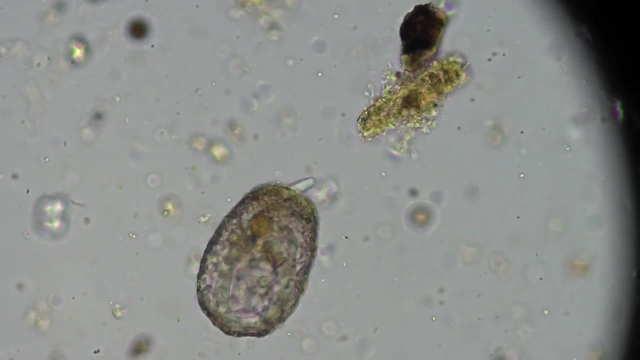 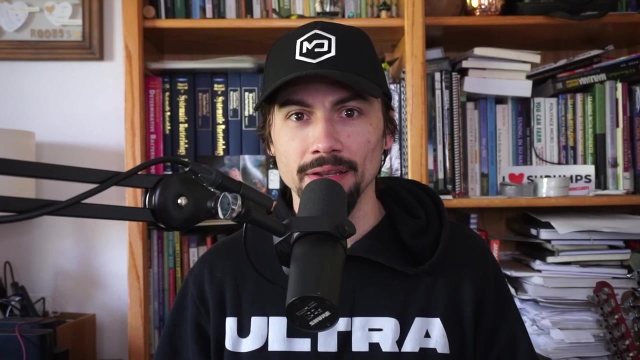 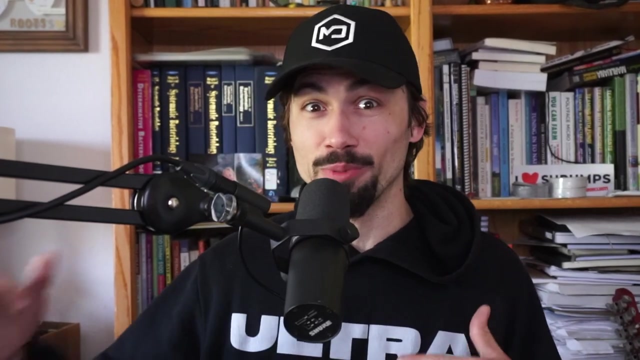 Yes, There, there's something going on here. Yeah, This is something I've never seen before. I've known about it. People said it. I've never seen them share any footage of that, Any of my mentors, any of my teachers, in any of the books and any of the videos online. 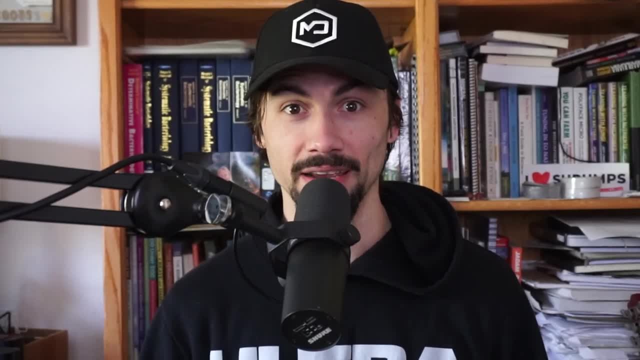 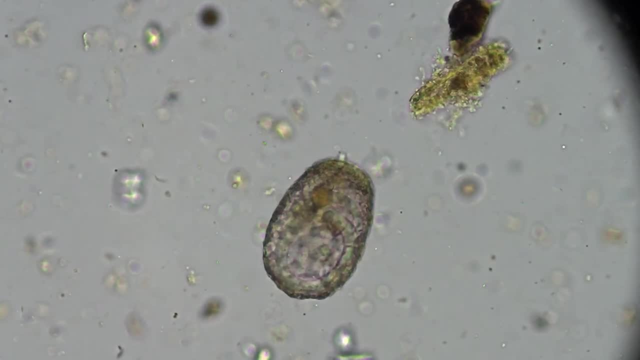 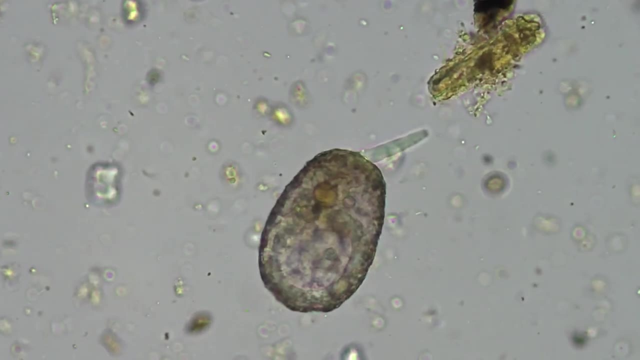 anywhere in the world. I've never seen it before And I've done so much research years and years and years on this space. And you can see its mouth parts. So it's- it's very obviously not a predator nematode. It's not. 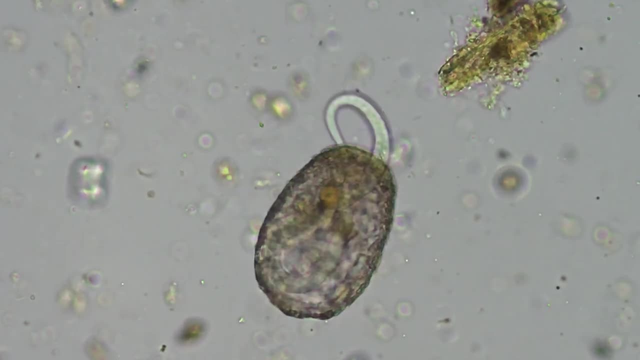 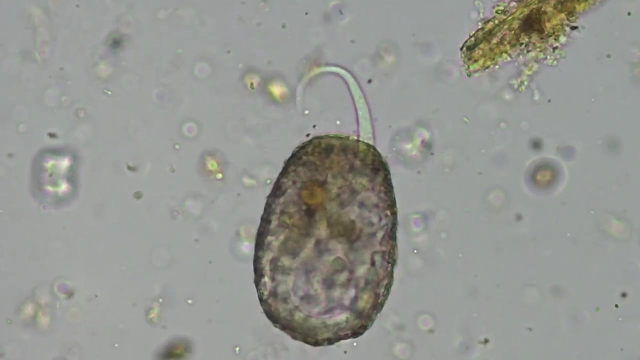 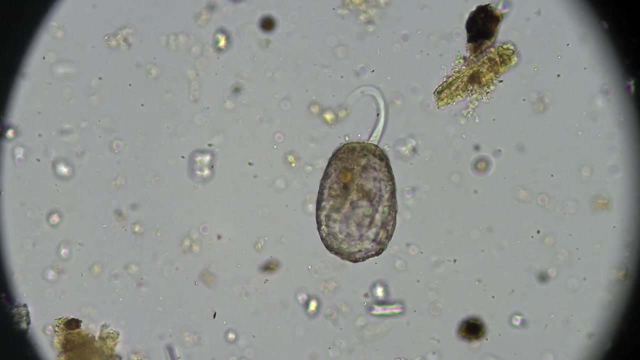 going to eat other nematodes. This is. this is an omnivore, maybe even a bacterial feeder, That's going inside of this testate amoeba and feasting Like it's this cornucopia bread basket for it to go feed in And whether it's damaging the amoeba. 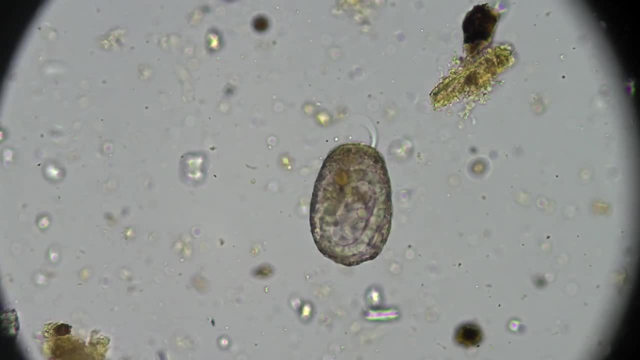 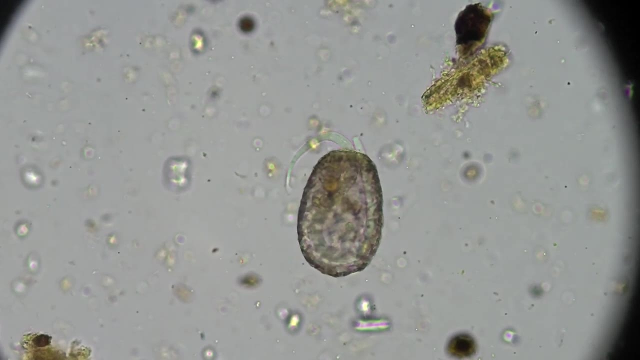 whether it's eating the amoeba- not very clear, But what we do know is that it's going in there, It's roughing it up, It is it's feasting, it's feeding And it's it's it's it looks like in. 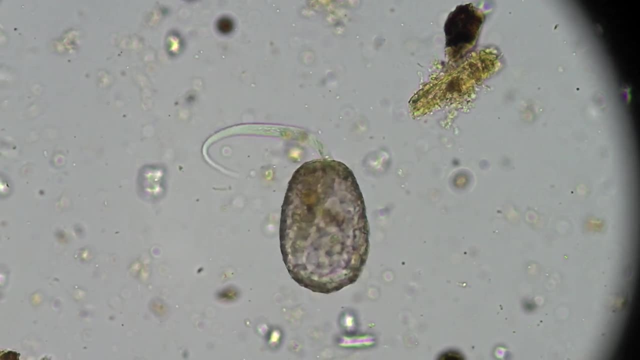 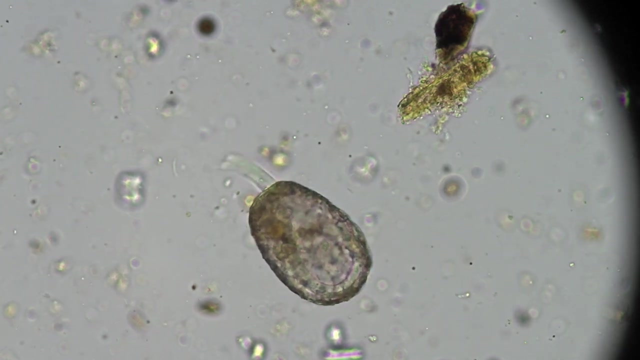 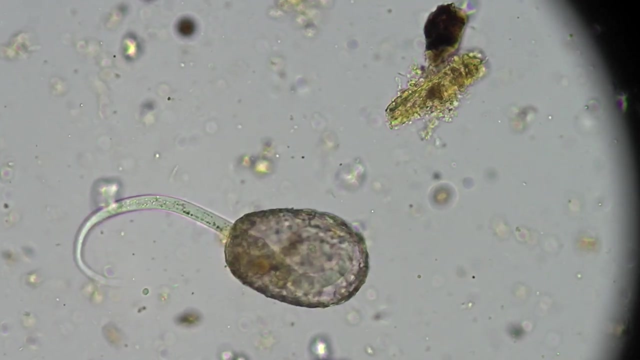 its action it forced out some of the bacteria and that's why it pokes its head back out and grabs things that came out. Obviously, when you have a large testate amoeba with a giant mouth opening, it's going to be inviting to a nematode, especially if their food source is inside it in a large concentration. 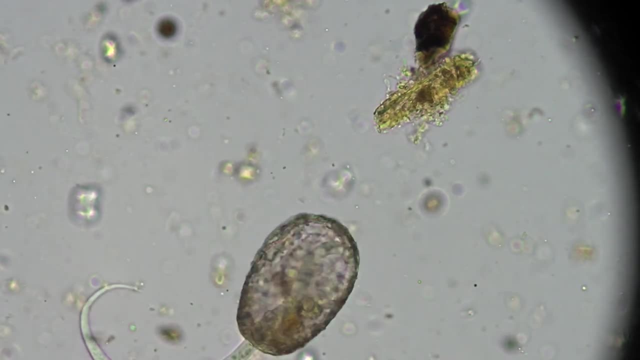 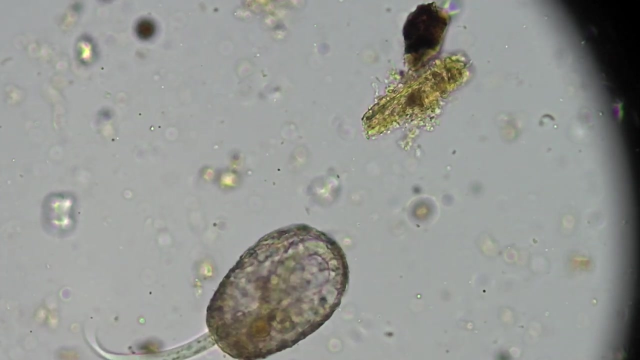 And it's going to seem easy, you know, for them to go in and out. It's going to seem really tempting. But there's another aspect here. When we look at these testate amoebae, they, they, they all look um sessile. They look still, They're just going to just 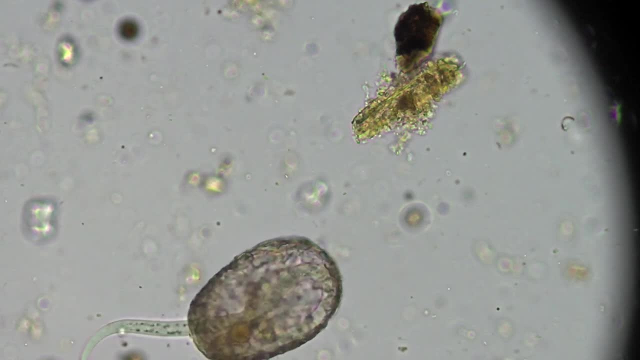 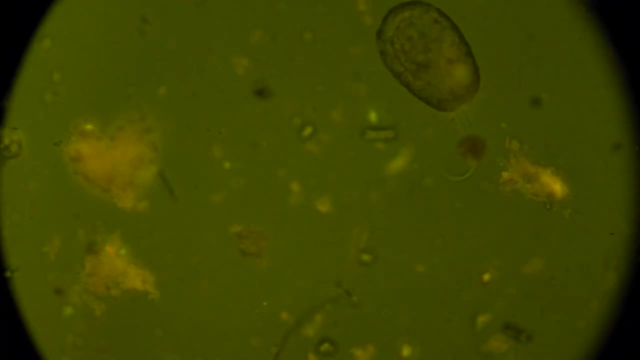 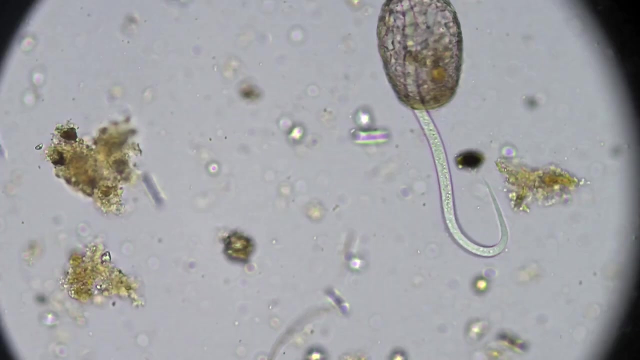 be moored onto something, Um. but then at the end here we notice that there's there's kind of a little bit of a drama. We can see that the testate amoeba is somehow holding on, And then we see its shape as it gets flipped around by the nematode as it tries to escape. 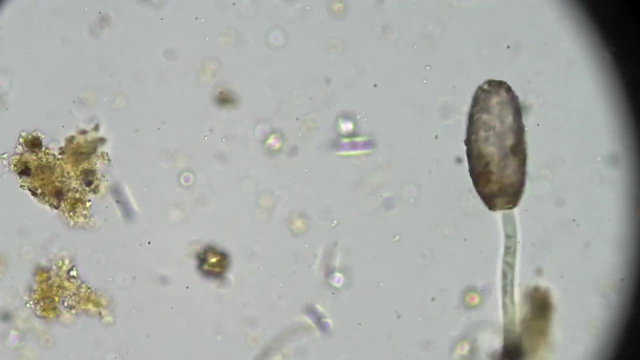 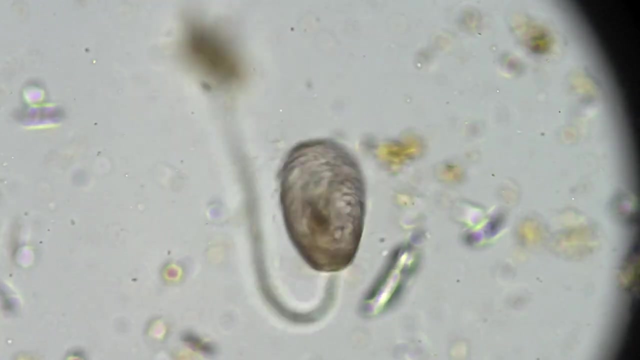 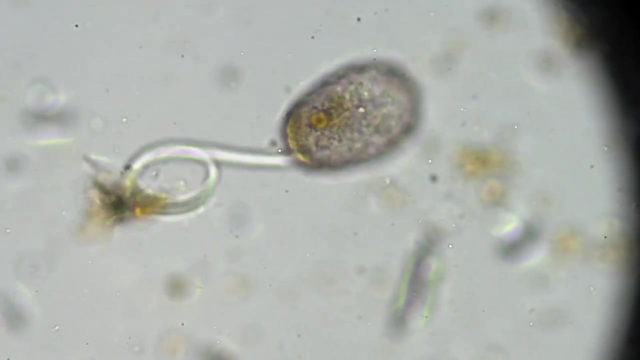 So, yes, it did feed on it, but there seems to be a reaction here. There seems to be something going on here. What is it stuck on? And? and then we see the shape: It's like a clam. This testate amoeba is large and it looks like. 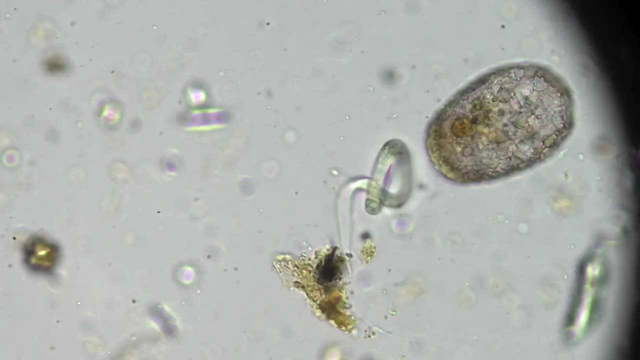 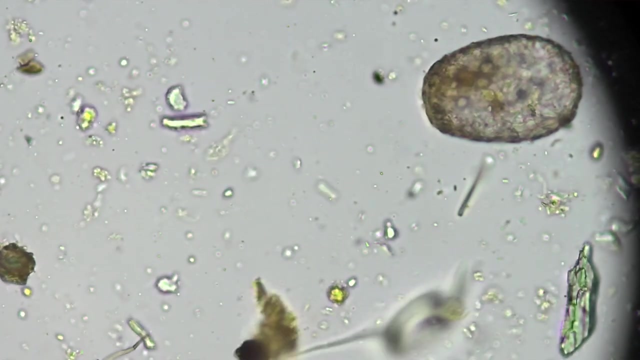 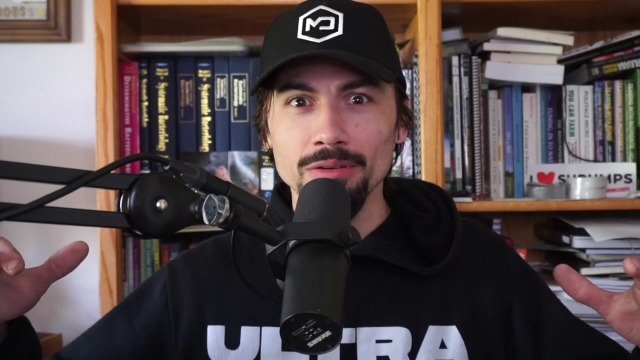 maybe it was able to close its mouth. Not, we're not clear yet, but this is the kind of non-definitive level cutting edge of the reel that we're at right now. This image, this video, this is the kind of non-definitive level cutting edge of the reel that we're at right now. 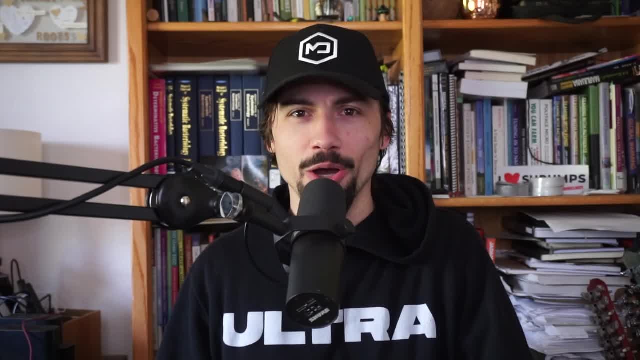 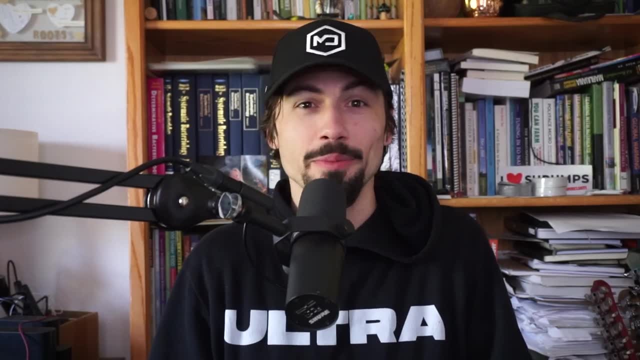 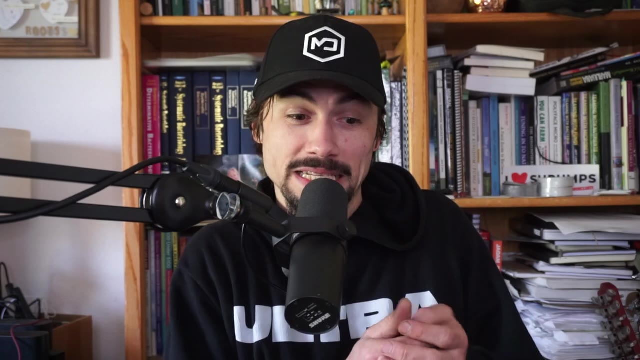 This is. this is a sample of catalyst bio-amendments- hot thermophilic compost that they age until it's just right, And it's, they're amazing. Keisha and Casey are amazing, Uh, and it always delivers. And I I shared this with them over my cell phone, with the cell phone video. 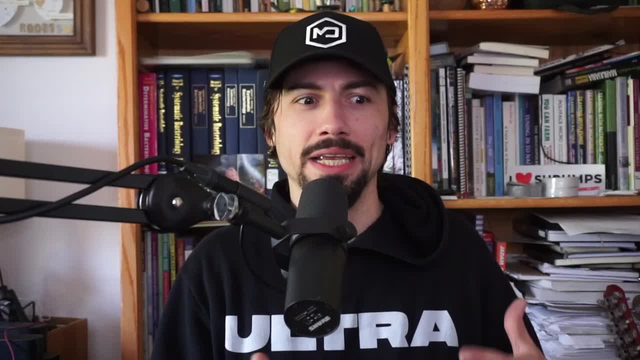 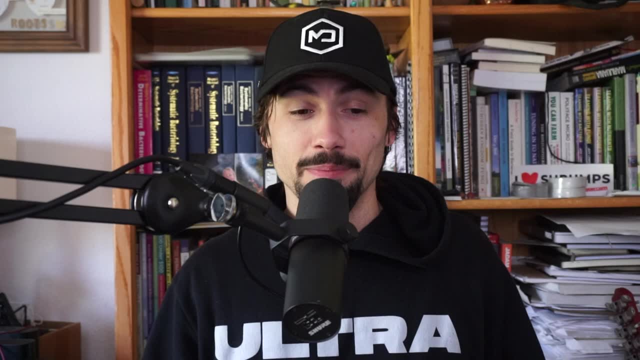 of this video, as I was, as I was looking at it for the first time, and they immediately shared it. So maybe you saw it on their feed, a clip of this, but but this image- before this they didn't have an image of this. 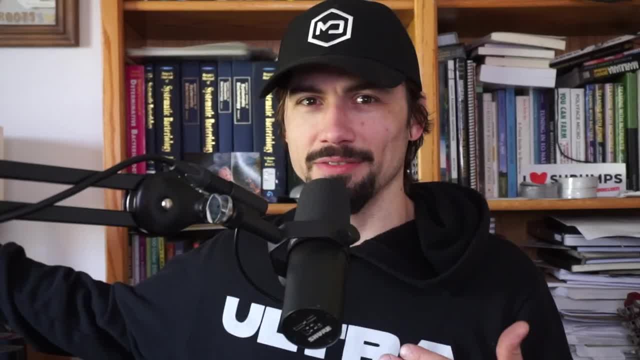 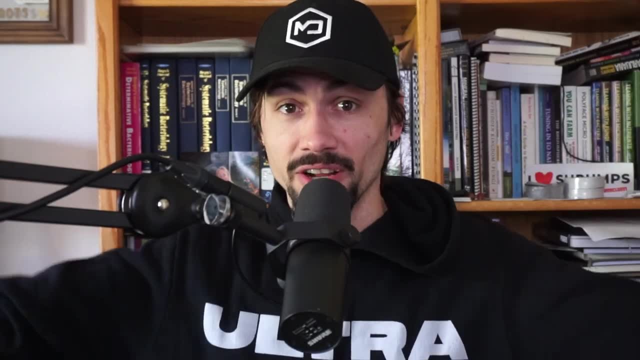 Our mentors didn't have images of this. None of the books. I've ever read any of the studies online, all the published studies that I've paid for, the books that are over $500 each that I've paid for, none of them had this image. So what I'm sharing with you today? 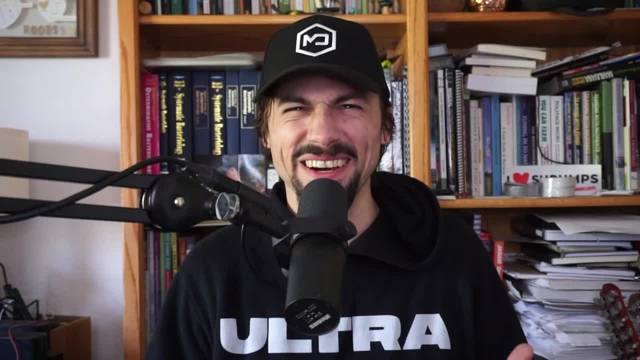 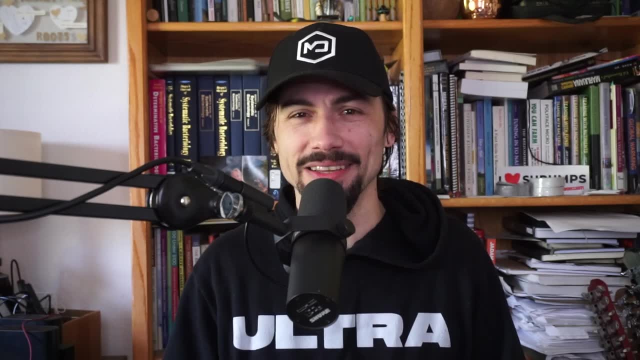 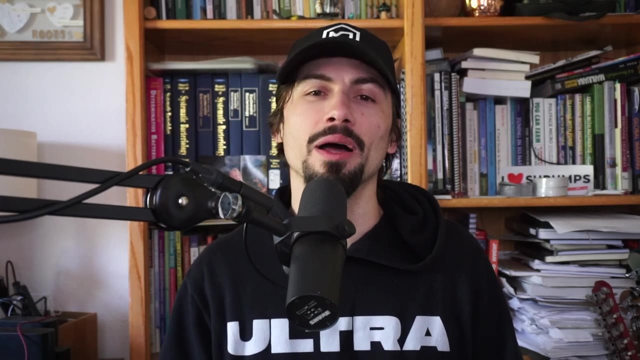 has incredible value And it's also a groundbreaking moment in soil science. So I wanted to share that with you. I want to bring you that high quality- 4k quality- and share with you what's really going on in the invisible world, the world that we all rely upon, because healthy soil is the key to 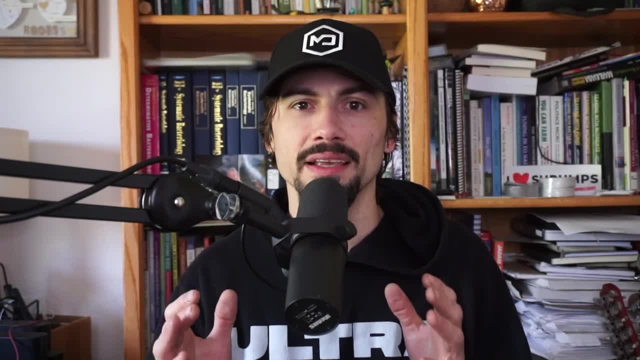 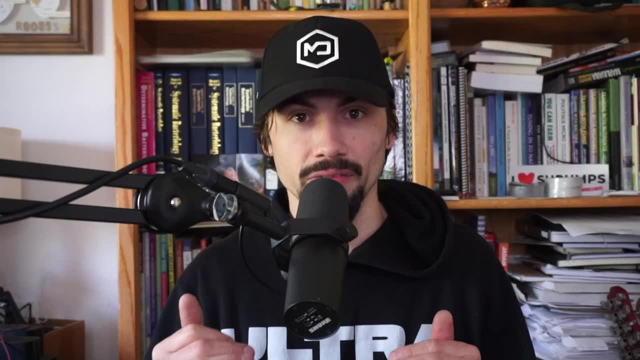 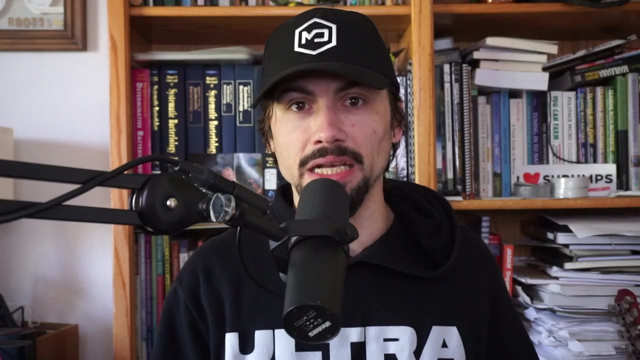 healthy plants, and healthy plants is the key to healthy animals, And whether you're eating those animals or eating the plants that your health depends upon them. you know no workout, no physical regimen will ever make up for a bad diet If we're poisoning ourselves with the food. 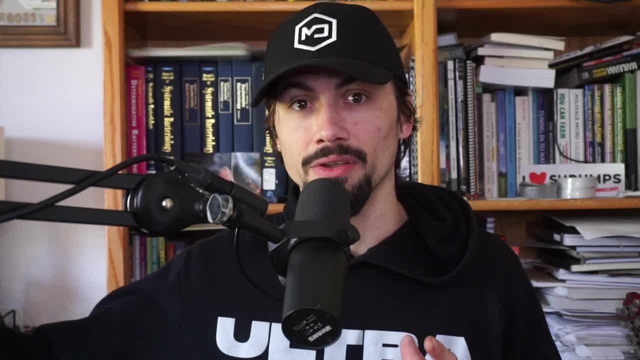 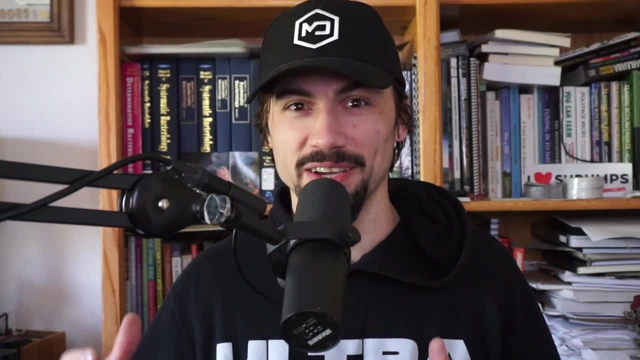 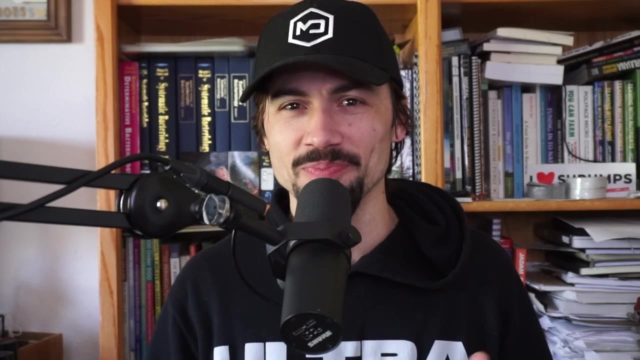 that we eat. it will affect everything in our lives. So we have to do better. We have to fix our soil so that we fix our food, so that we fix our health from the most primary, fundamental space, And that's what regenerative soil is all about. Thank you for being part of this community. I'm 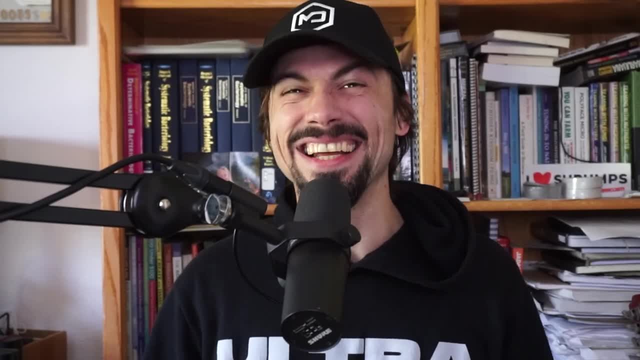 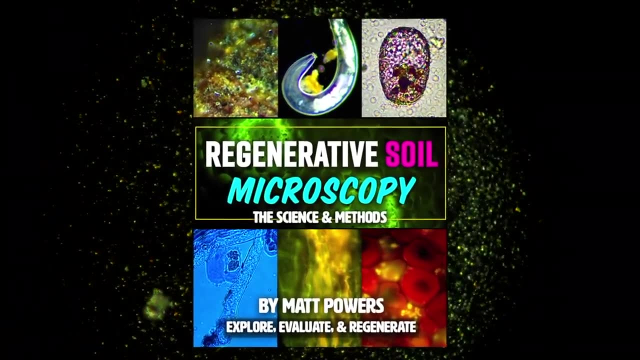 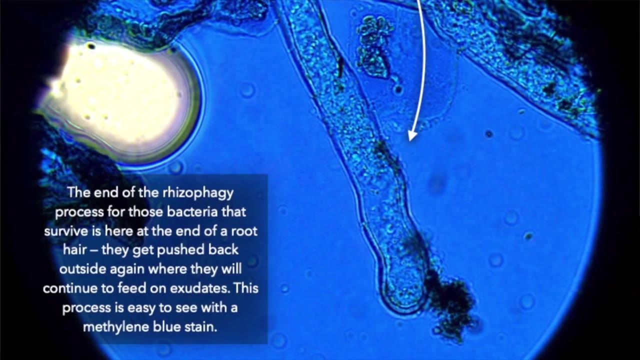 Matt Powers: Grow abundantly, learn daily and live regeneratively. And check this out. Regenerative soil microscopy is the first soil microscopy book of its kind ever available. Focuses on the soil biology, compost, mycorrhizal fungi, rhizophagy. 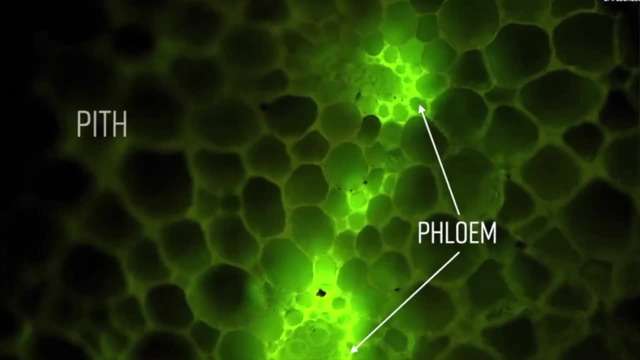 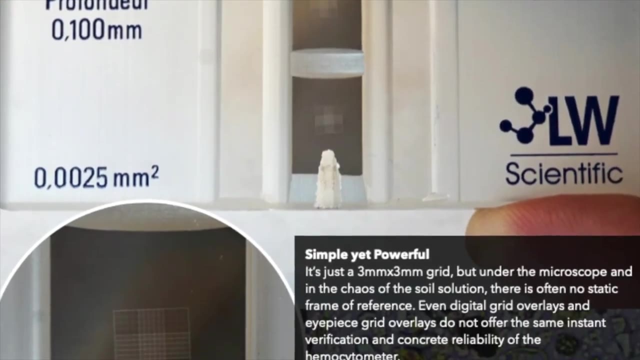 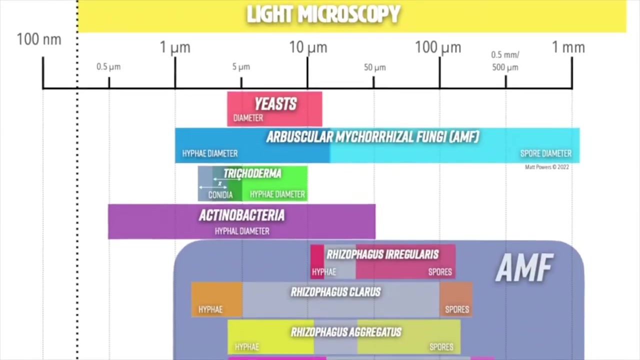 and so much more. That is the life that makes all of our plants nutritious and healthy, And it's also a how to, how to operate the microscope, how to do stains. the recipes, the directions, the step by step. that's all in there, But not only that. there's a morphological guide, so you 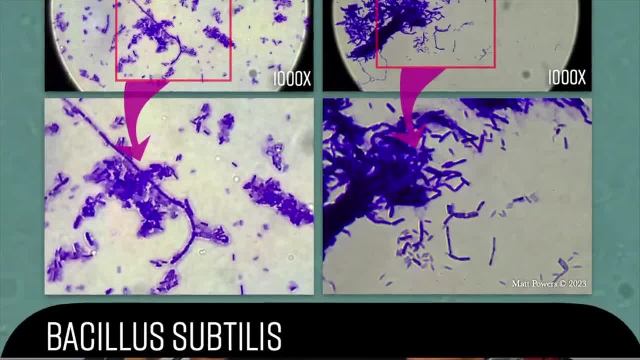 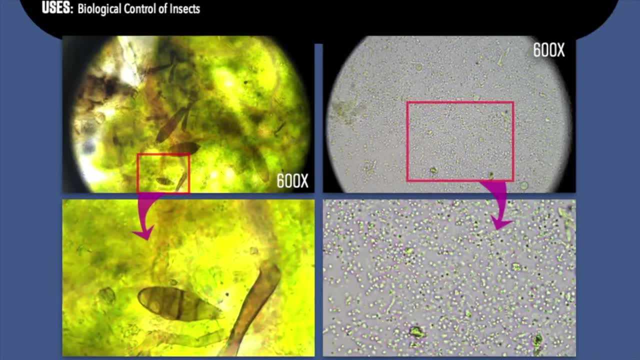 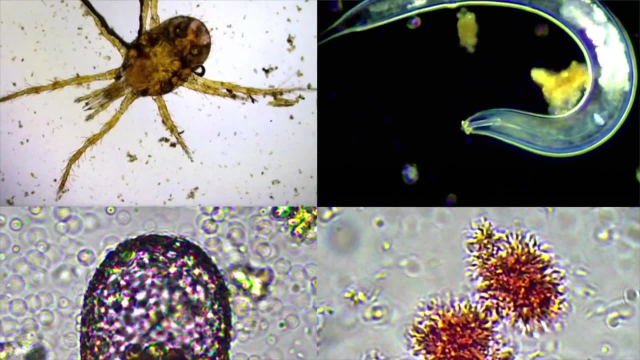 can compare what you're seeing against proven, lab certified samples. So this is a game changer. This has never been offered before If you want to see examples of the fungi and bacteria that matter: the protozoa, the nematodes, the macro arthropods, the micro arthropods. 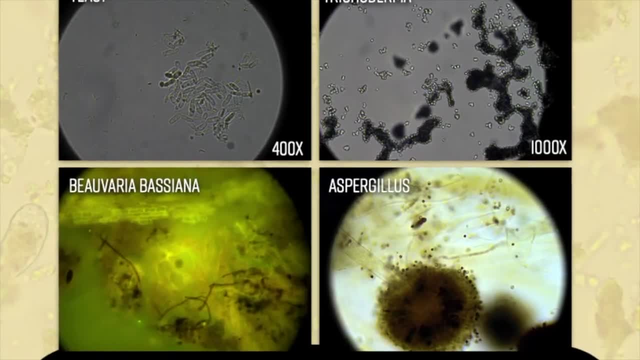 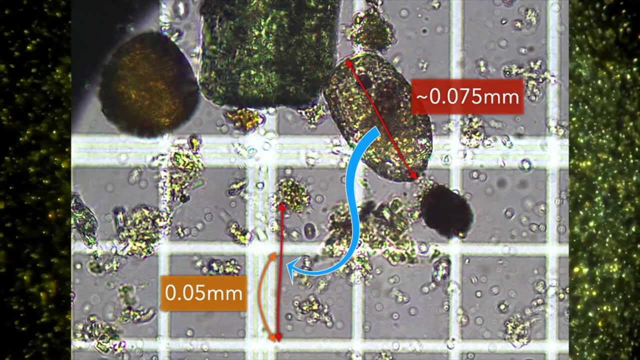 all the soil microbes, all the trophic levels. You want to see examples of them, You want to be able to compare them. You want to be able to look at the mouth parts. You want to look at the gallery of images so that you can sharpen your eyes. so 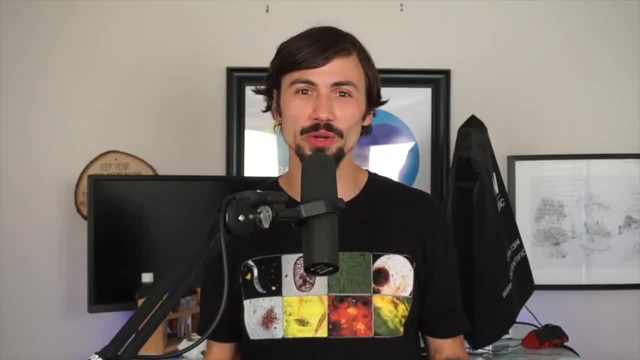 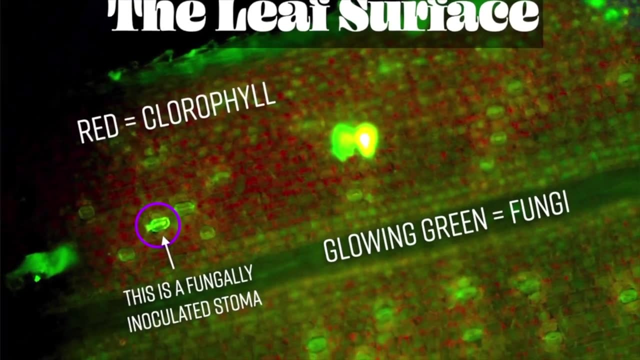 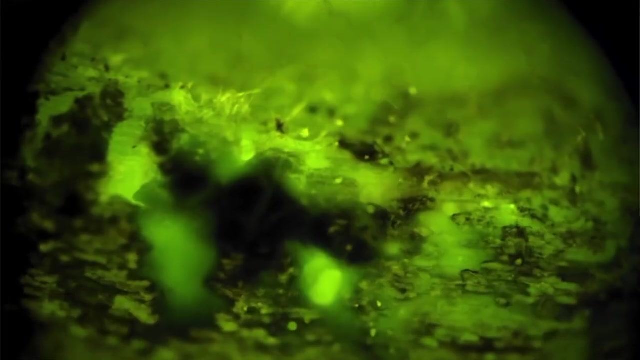 that you have a reference of comparison as you travel and explore soil, compost, indigenous microorganisms, even roots and plant leaves. We cover it all And it goes beyond bright field, So it's dark field, It's epifluorescence light, And so you can see the invisible fungi. You can 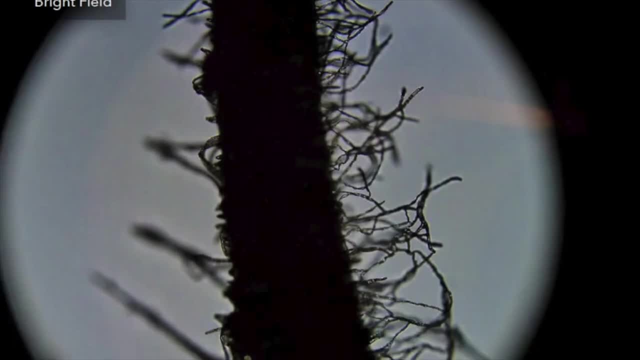 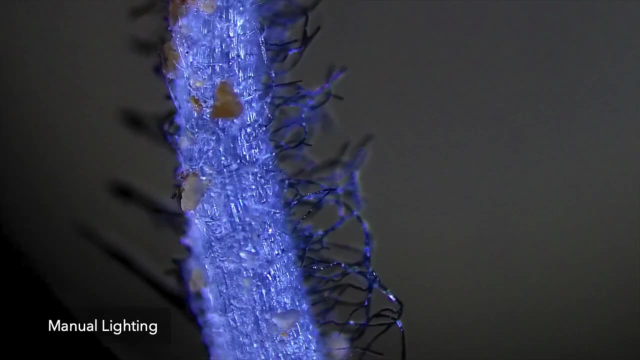 see the phosphorus where it goes and where it glows. Also, manual lighting, which is a new creation that allows us to visualize roots and plant surfaces at a completely new level and allows us to see them in a much more natural and understandable light. 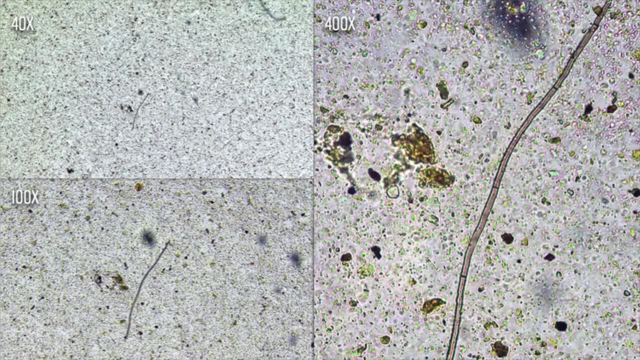 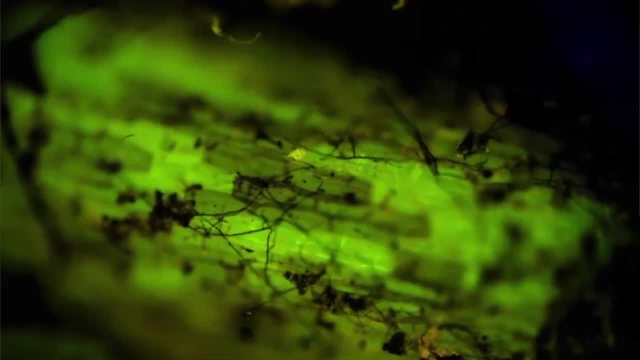 If we don't look, we don't see. If we don't look through multiple lenses, we miss what is otherwise unseen. Mycorrhizal fungi is invisible in bright field. microscopy, New methods, new interpretive keys, new insights, new. 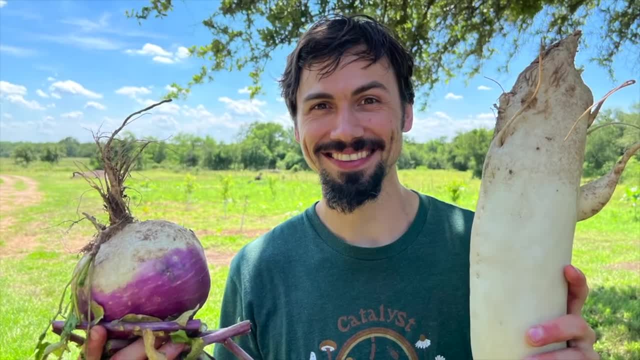 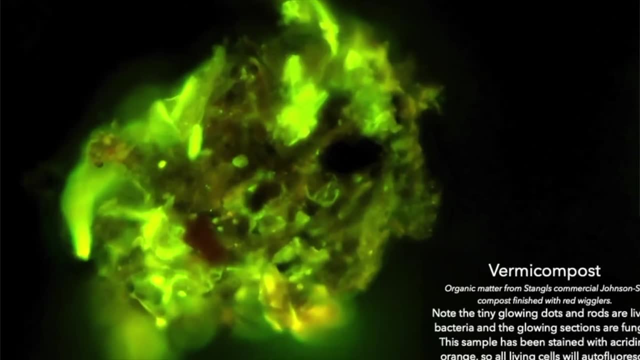 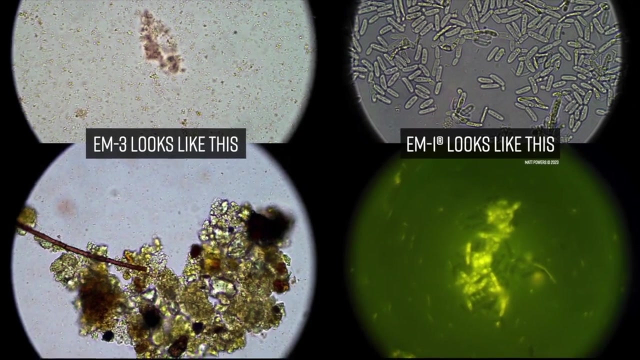 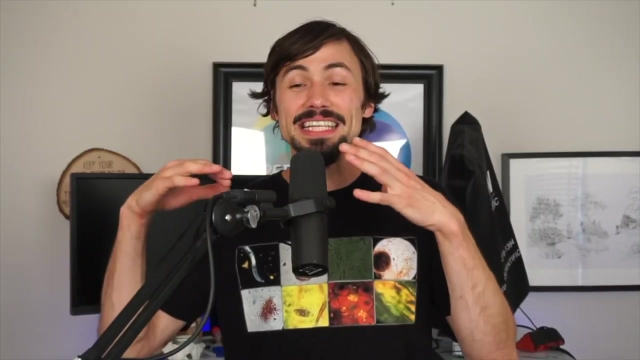 discoveries and next level results. We even have case studies comparing Johnson Sue to hot composting, to vermicomposting, to dead sandy soil, to a compacted dirt road, effective microbes, comparisons to EM1, EM3, to bruise of purple non-sulfur bacteria and even collections of 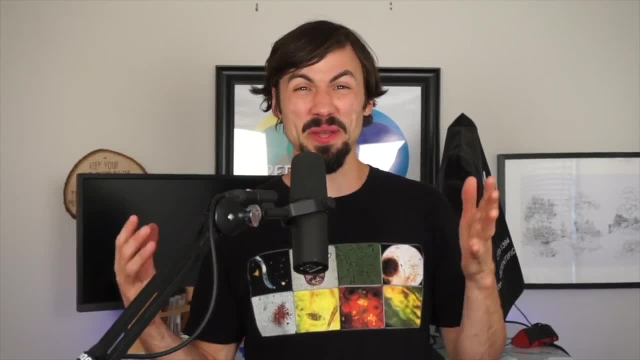 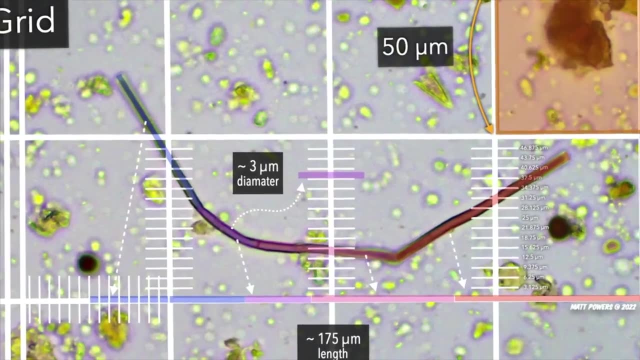 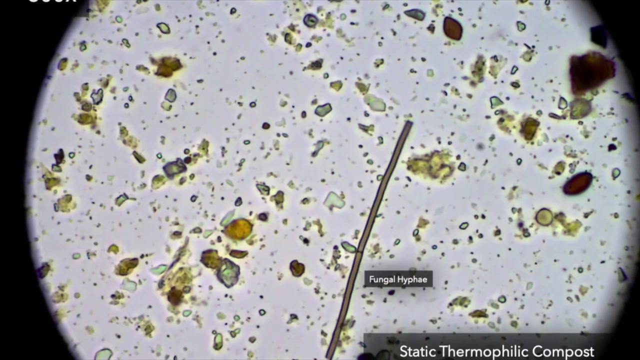 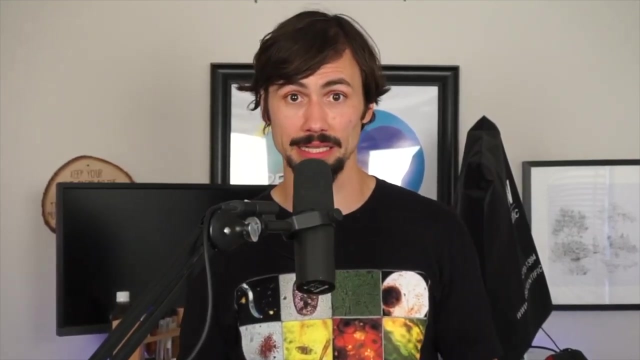 indigenous microorganisms. We look at them all and put them all together in this book. There's case studies, There's how to learn how to do the microscope, but also there's morphological guides, There's sizing guides. There is so much information in this book that has never been available, ever in one place. 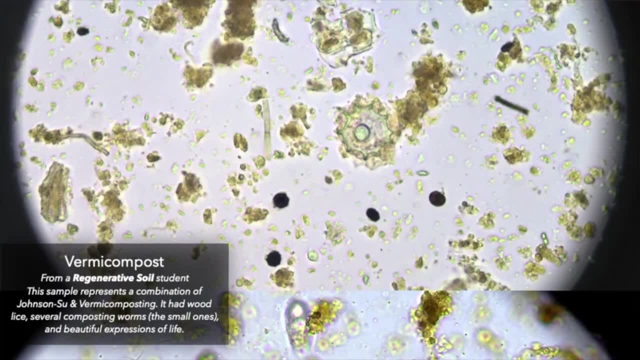 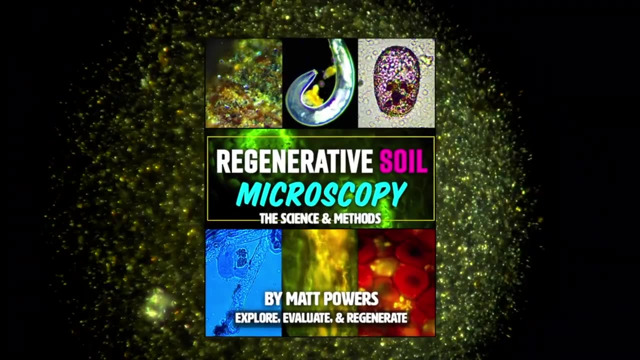 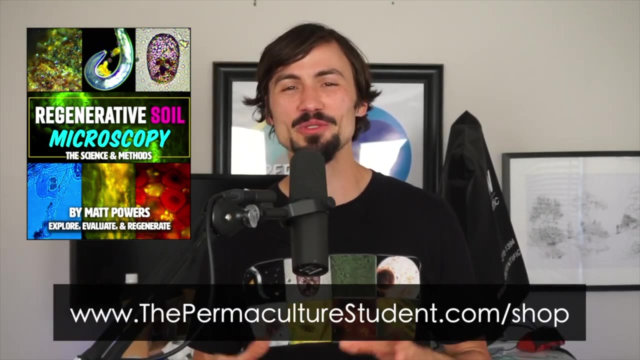 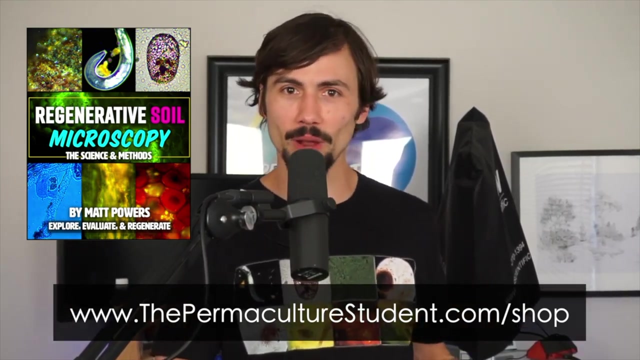 So compare the images to the tests and see for yourself. Get all the data, all the images, all the sample types all in one book. Order your copy today at ThePermacultureStudentcom. Thank you so much for being interested in soil and soil microscopy, because this is the only way.